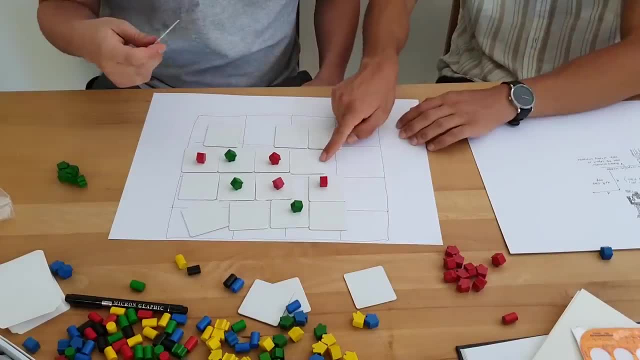 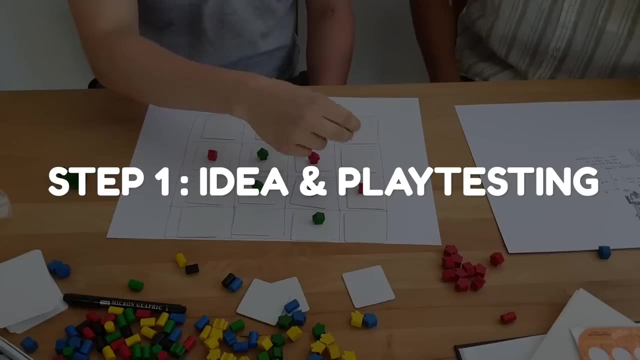 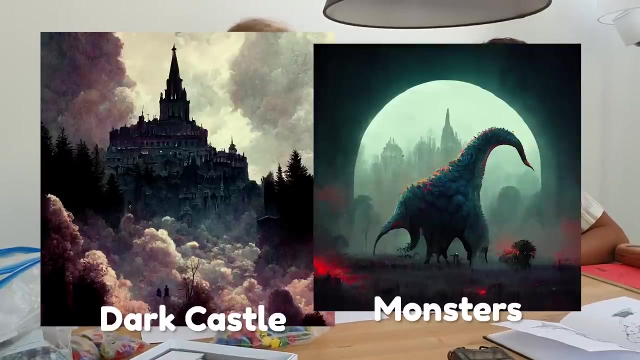 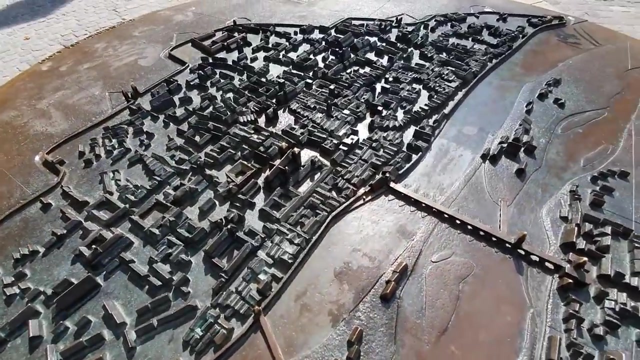 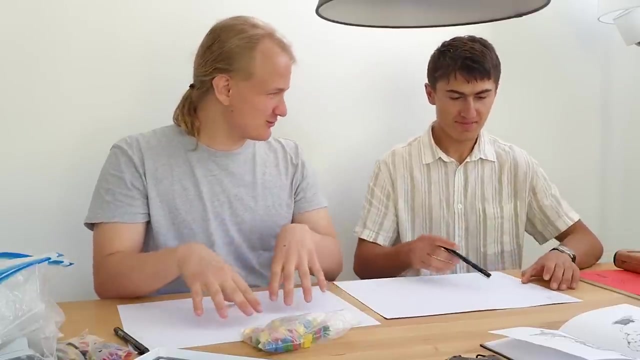 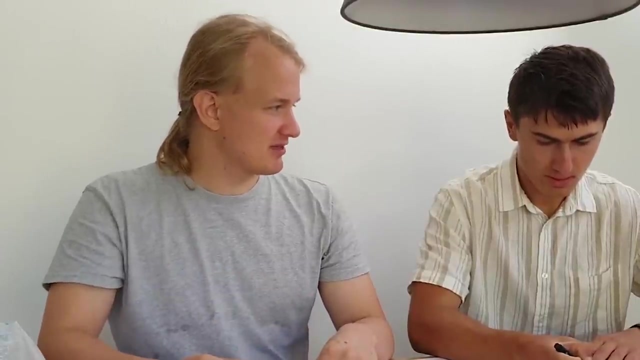 simplicity, because there's no programming or complex software. So here's a short story of how we created our game Townshift, from the early idea phase all the way to the final playtest. It's a puzzle game where you have to fit them on a map or something. 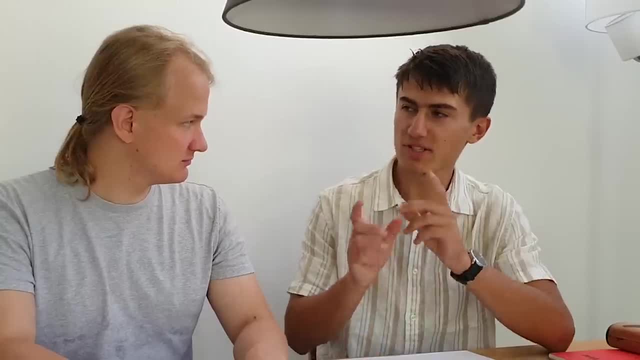 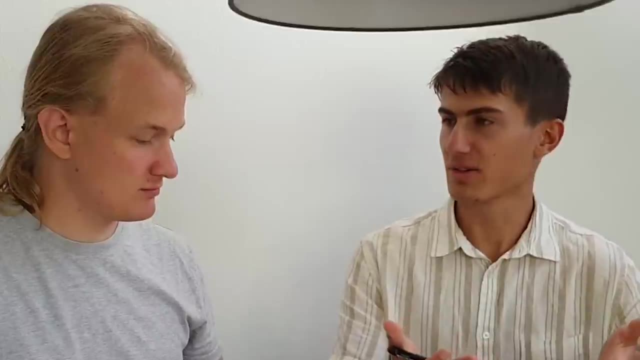 It is a placement building game. okay, It's kind of like a versus mode as well. You've got to fill out every square with a building, but to make that harder, there's me attacking you at the same time, or like shifting your squares. 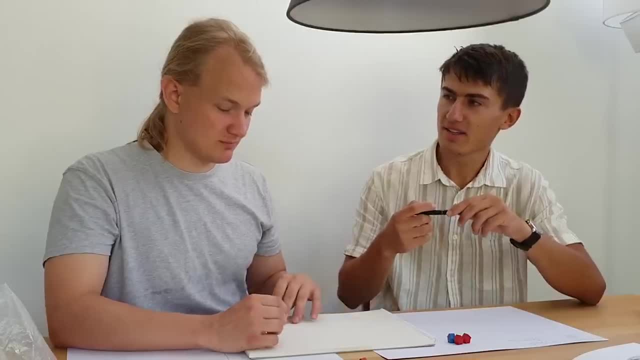 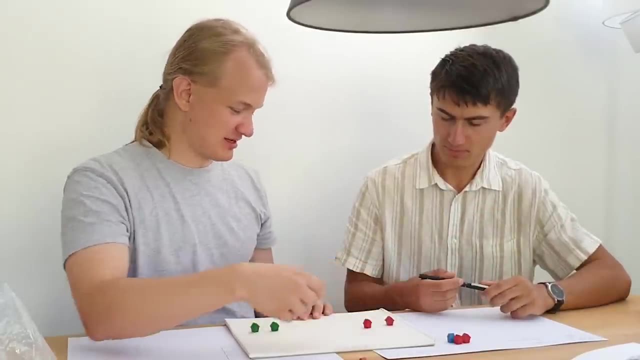 or moving your houses around with cards. But there are two rivaling villages and you're kind of trying to build in a way where you cut the other one off or sneak past them. So it's a versus mode, It's a versus game, right The end goal, the win state. 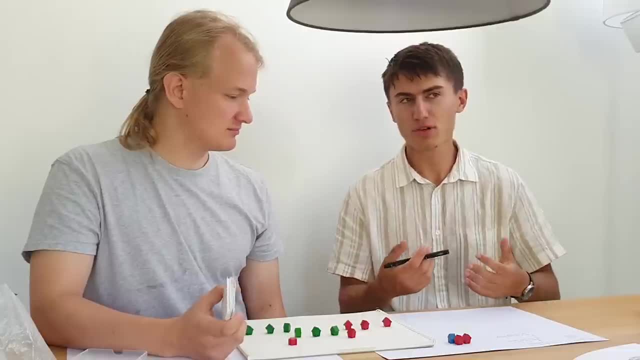 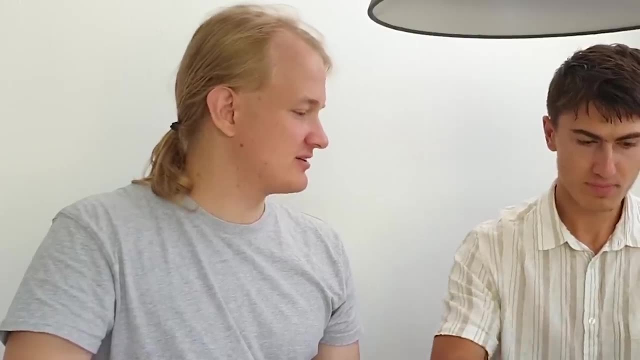 is filling every square with a building, So every turn you can place buildings, play cards that are going to shift the terrain of the opponents and make it harder Thematically, how does that fit into the fantasy of building a city? It's a fantasy-like city. 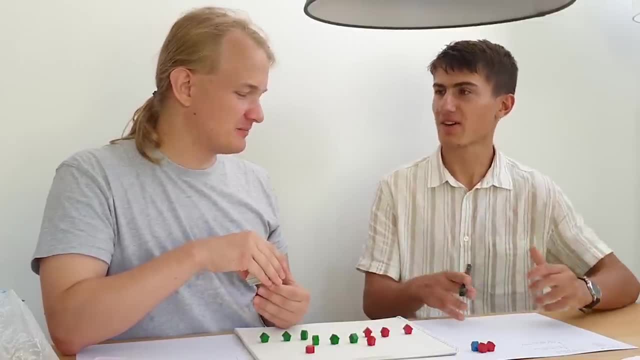 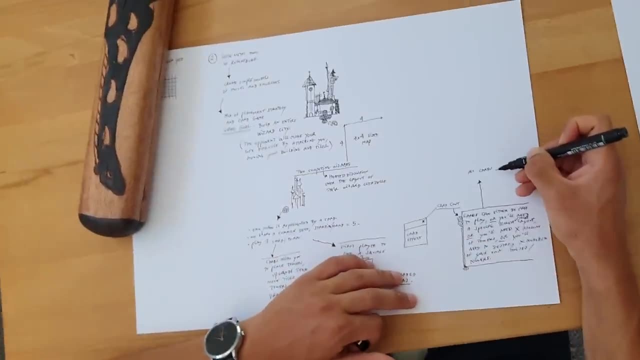 City in the clouds, or yeah, Exactly. yeah, It's a wizard citadel or something. I feel like the first thing we should really try to focus on is getting something playable Exactly, And then, as step two, we'll try to make a nice-looking version. 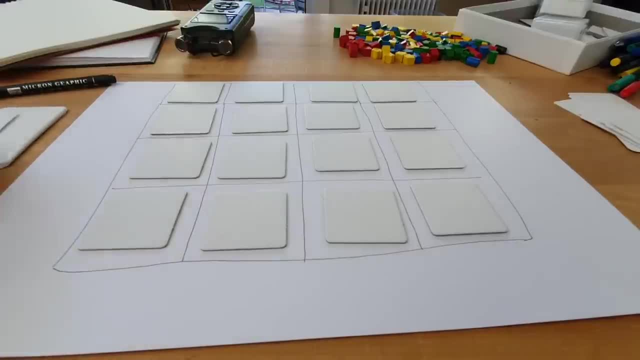 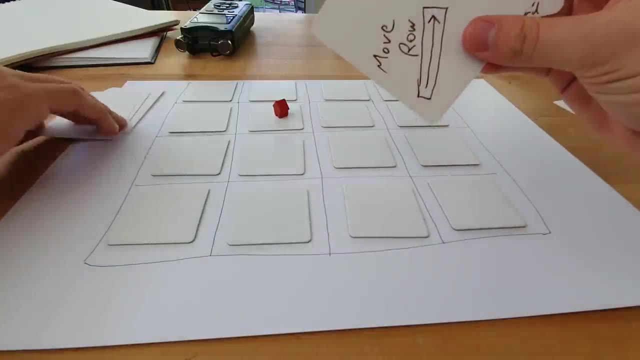 Of course. then we'll have to look up clay garden Playtests recording eight, four, nine. What if I don't have any card that places a building? So first we'll just draw a card and I would say: True, I'll draw. 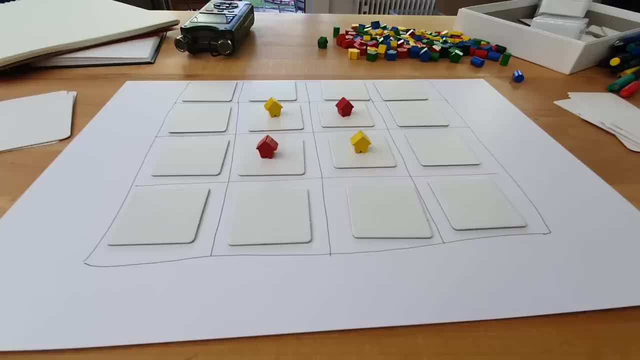 I'd say we need a lot of building cards. Maybe place building should just be a default option that's always available. Yeah, exactly, You either play a card or place a building, which is cost and action. I like it because then we can also put more interesting stuff on the cards. 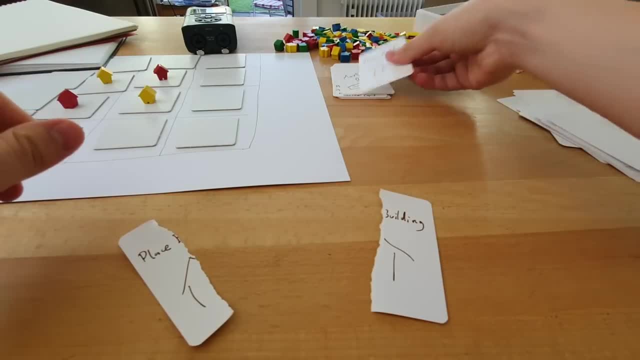 Yeah, Like place building is not an interesting thing. Exactly, if it's not a place building, we're gonna have to have like at least half the deck place building. Yeah, And it's not cool. Try and think of the most unique cards possible. 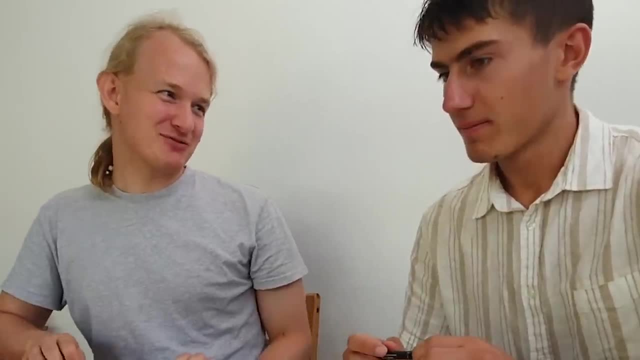 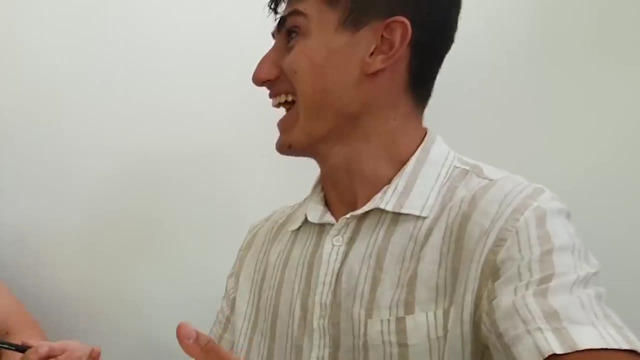 Then we just see which ones are good, which ones are bad. Slap your opponent in the face and if he survives, Yeah, If you knock out your opponent, you win the game. As a win condition, as a victory condition, Yeah, so we thought about making some random win conditions. 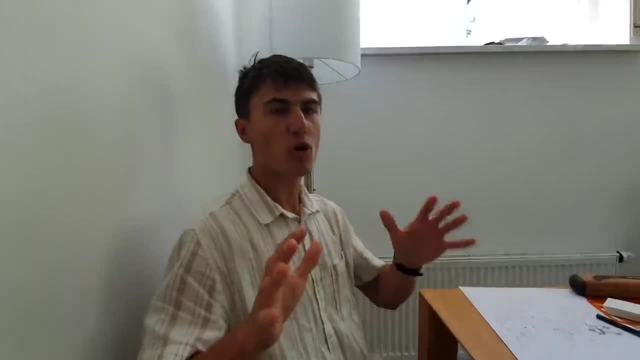 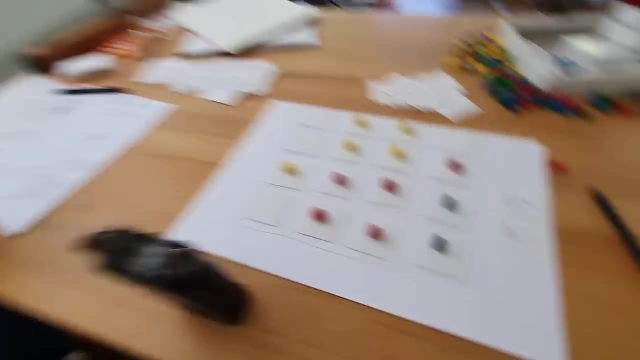 So every time you play you have a different win condition. Right, No longer win if you've got like a group of four buildings. You know like two by two, That's no longer the win condition. The game ends once the complete map is filled with tiles. 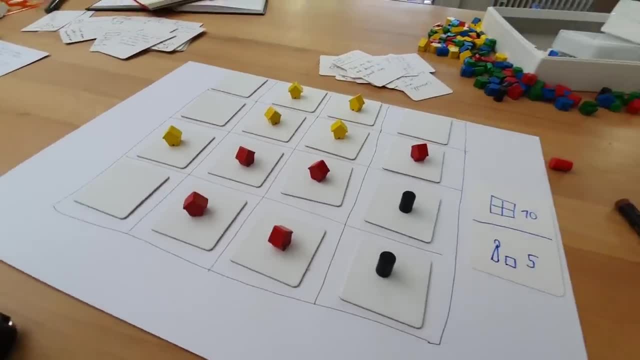 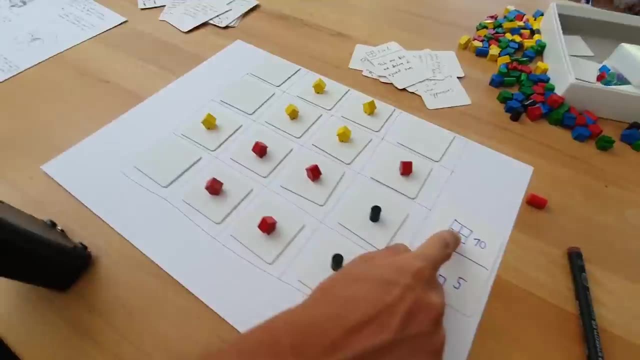 Be it neutral tiles or your tile enemies, And there's like a point system here. So, for example, in this example, you get 10 points every time you get a square, And also five points whenever you've got a tower adjacent to a normal house. 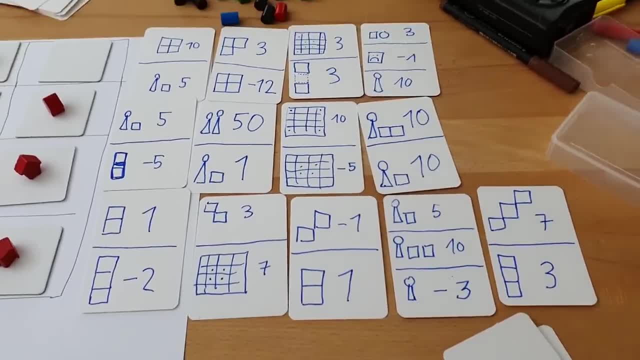 Yeah, we made a bunch of victory conditions, So it's not actually conditions, just like how to get points. Yeah, For a quick recap, each player is a competing wizard. At the start of the game, each player draws three cards. 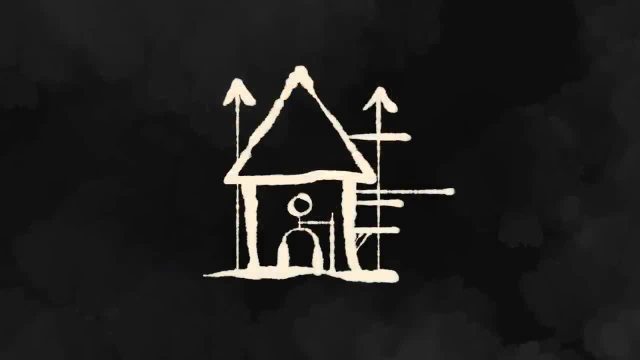 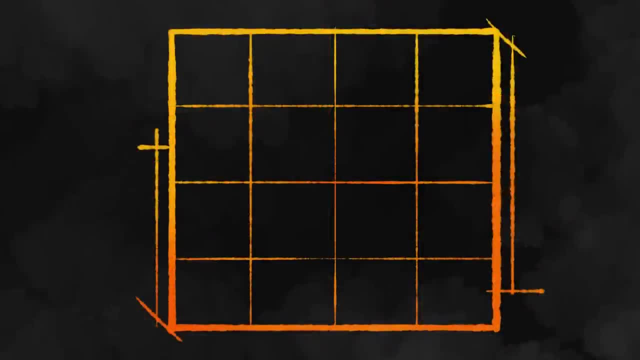 Every turn we draw an extra card. A card can help you build, move houses around, steal or counter your opponent's cards and, of course, destroy your rival's carefully laid out plans. Once you've drawn your card on your turn, you must place one house on the grid. 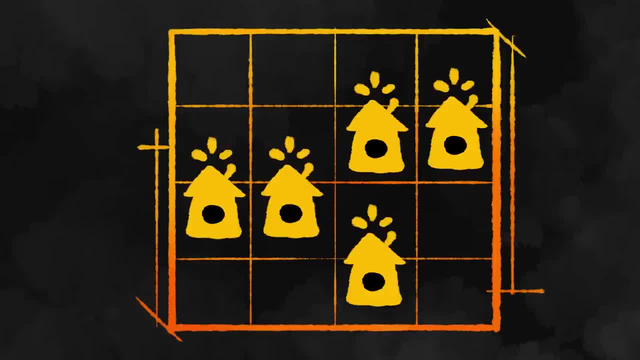 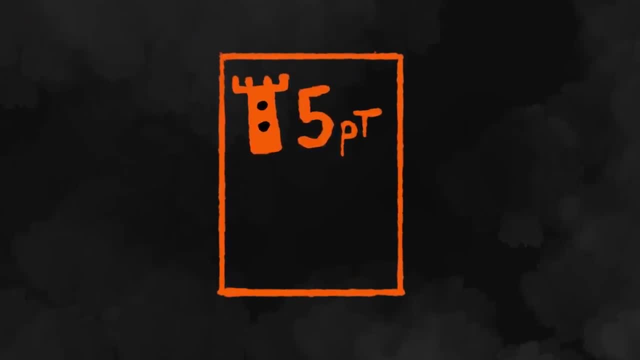 You can either place on an empty square or on top of one of your existing houses to create a tower. Towers can be part of the scoring system. For example, some rewards could be gained- five points per tower- but they can also help with the second phase of your turn. 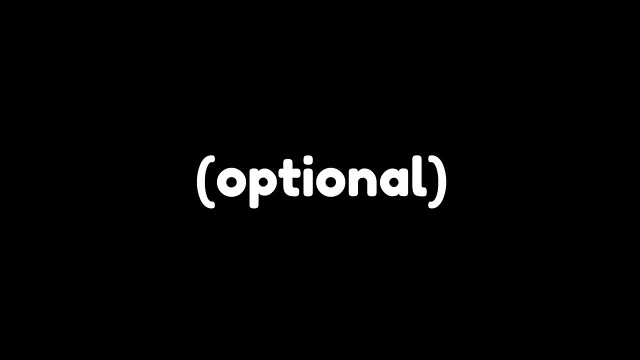 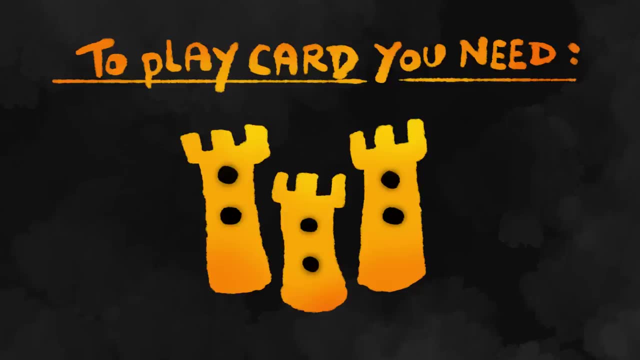 which is playing one card from your hand. This is optional. Cards have various effects and we made 40 unique card effects in total. Many cards cost something to be played. For example, to play a certain card you might need several towers. 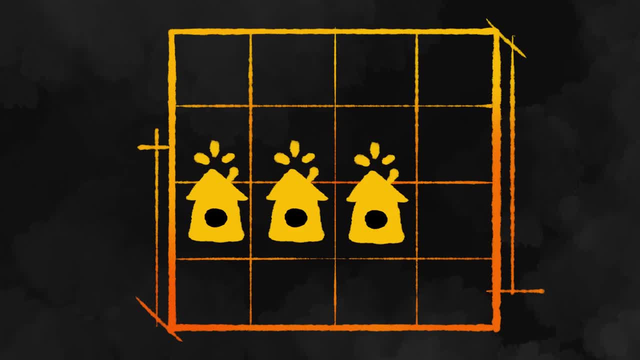 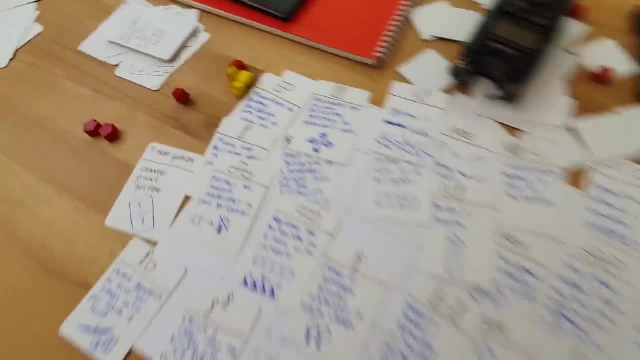 Or perhaps you'll need to discard a card from your hand or have three houses in a row. Some powerful cards even require you to destroy one of your houses or towers. Once all grid spaces are full, the player who scores the most points. 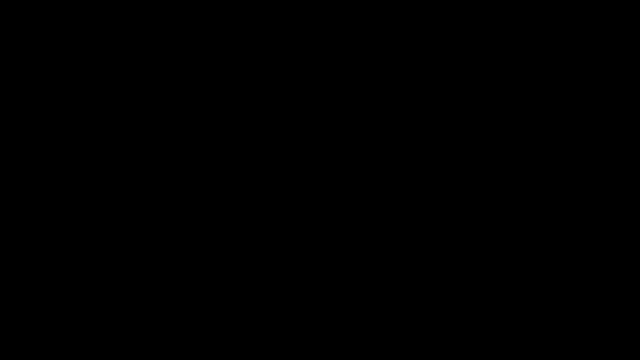 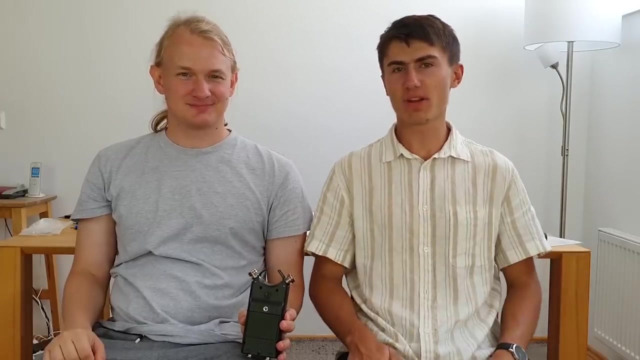 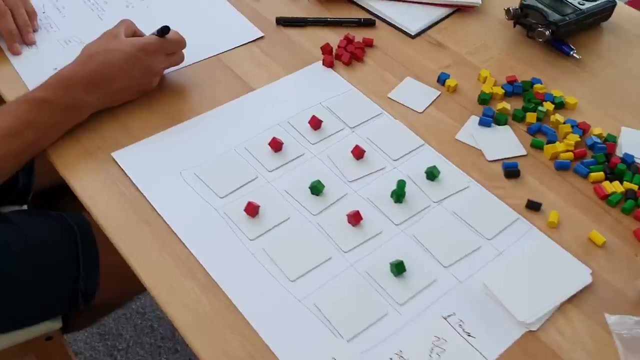 according to that game's specific point system, will win. So how has this morning been, Jonas? what do you think? We struck gold very soon. I feel like We got lucky. we definitely got lucky. We immediately came up with concepts we both kind of liked. 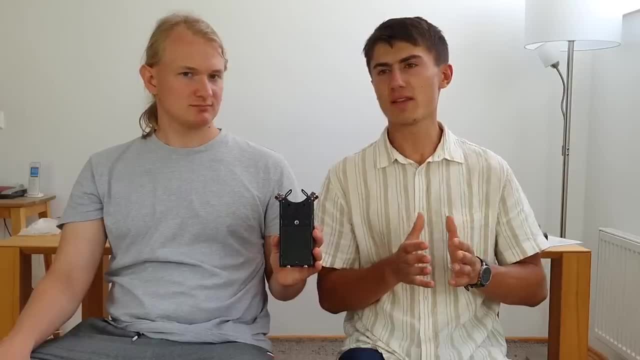 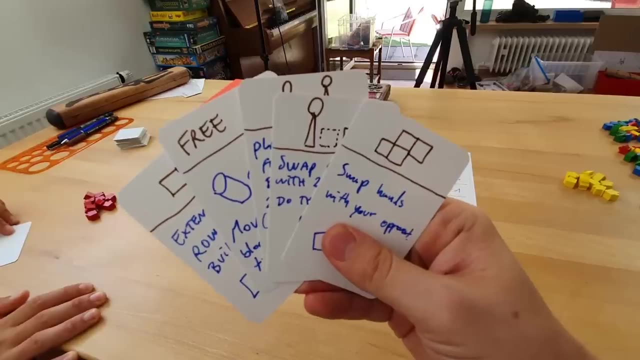 The plan this afternoon is to playtest what we've got, and after that the remainder of the day will be spent beautifying the creation, using the clay to make cool little sculptures, little towers. So we spent some time balancing the cards and mechanics. 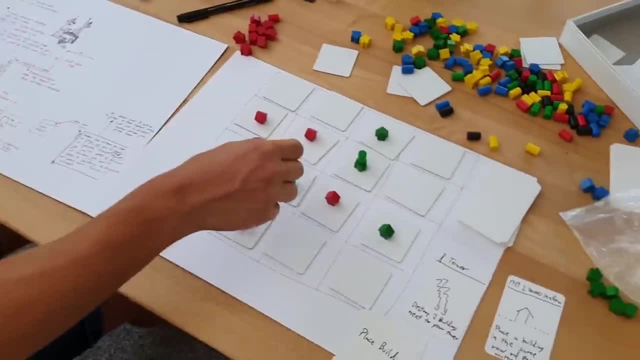 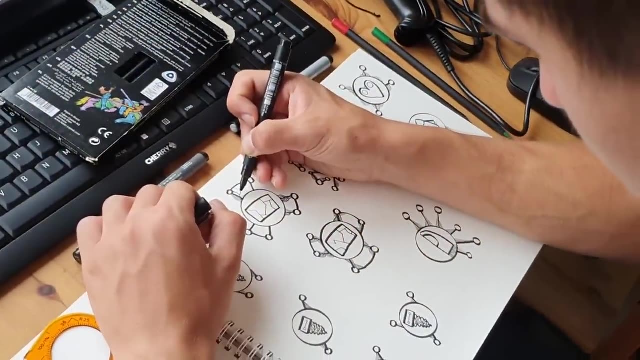 trying to simplify the rules whenever possible. One of the many things I greatly enjoyed throughout this morning was discovering Jonas's collection of excellent prototyping materials, For example, these solid white cards, When trying to prototype games surrounding oneself with simple good materials like large sheets of paper, packets of dice. 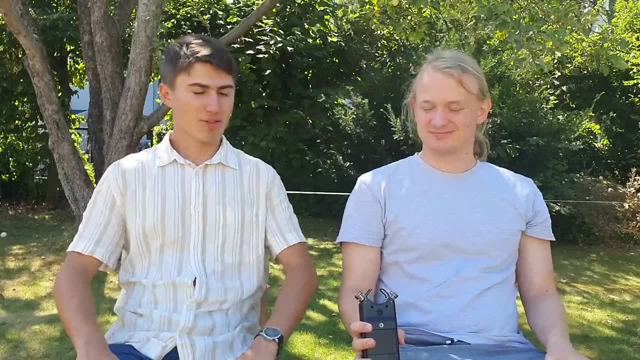 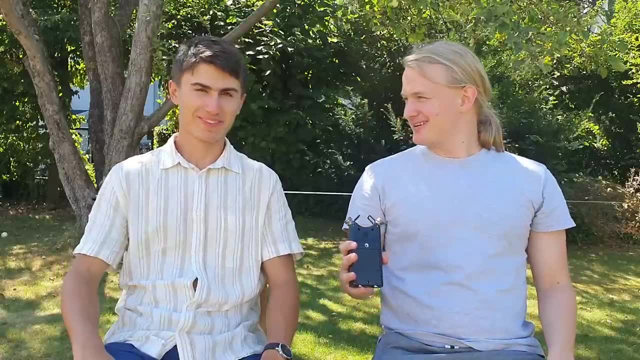 a whiteboard and a clean, spacious table could really go a long way. It's three o'clock now. we've got a couple hours left. and what's the good news, Jonas? The good news is we got the gameplay pretty much figured out. 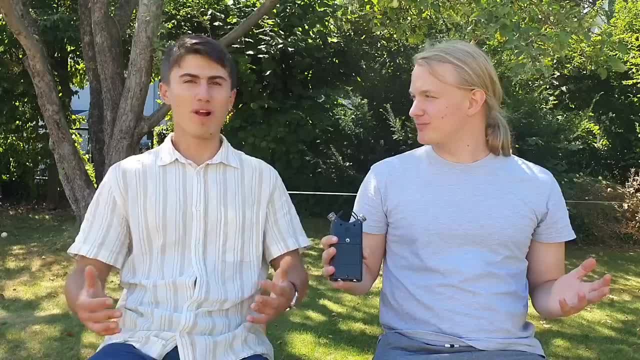 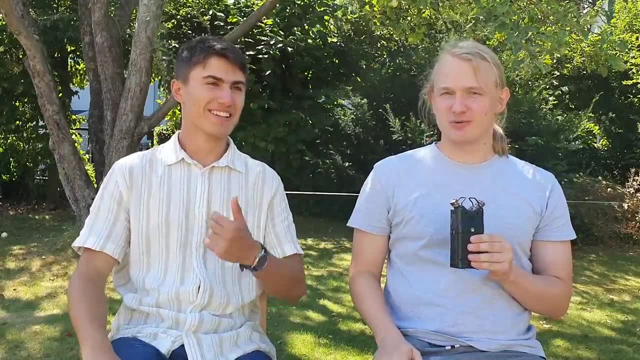 we have a very well-working prototype that I think we both really enjoyed, Super happy with it. yeah, it's like it's all done in a couple hours. Congratulations, man. I mean I enjoyed it to a point. we both, I think, enjoyed it to a point where we 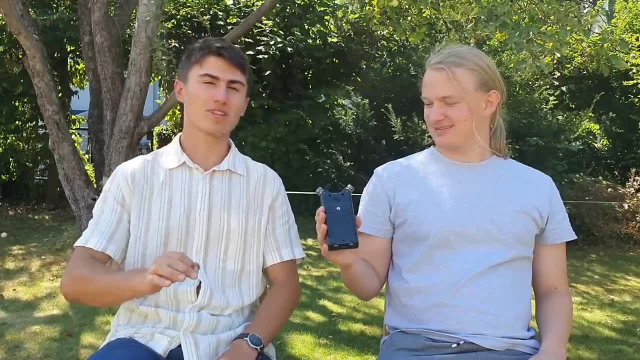 We wanted to play again. We wanted to play again. so that's a good sign. A lot of art to create. Yeah, Set a time budget for each task. We have the playing field, we have the cards and with the models, 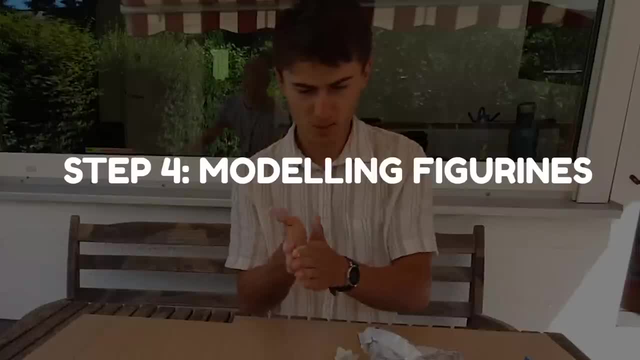 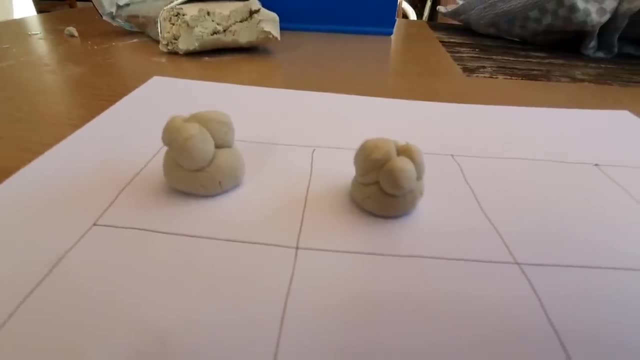 Three things. it's not too much And we have to paint the models Quite quite, quite agreeable, Quite agreeable to the touch. I like those bushes. these are looking good. they're also looking kind of leg-thornish. 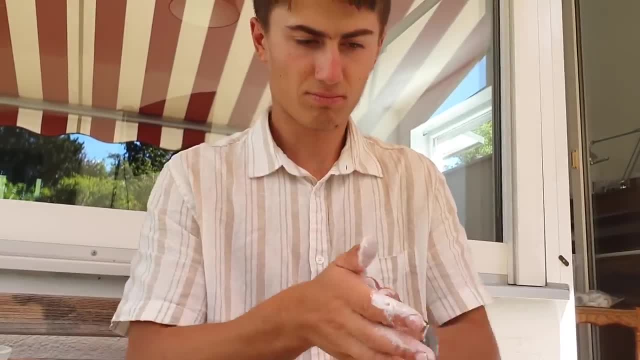 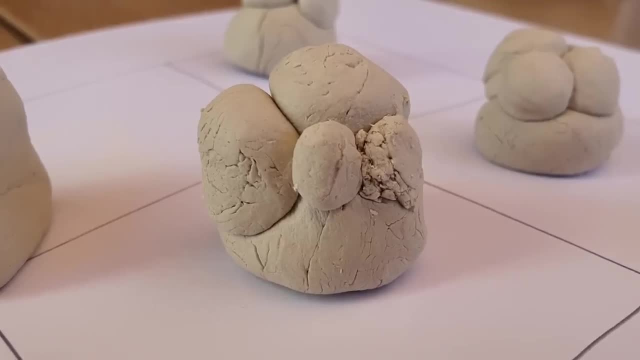 There you go, bake yourself. We began creating the models and, as we said throughout the process, we needed to be content with them looking rustique or just good enough. They weren't polished and if you zoom in too close they look pretty rough. 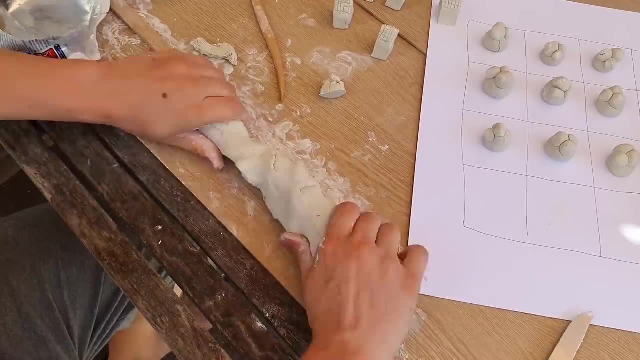 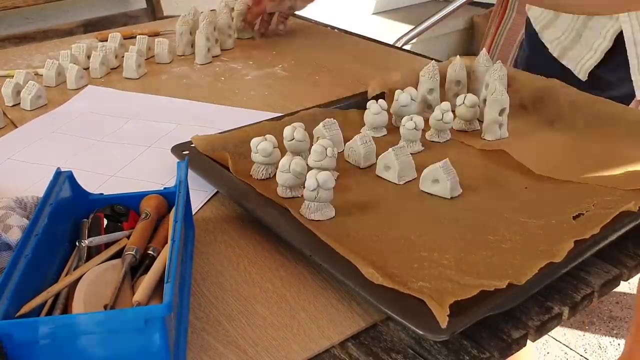 Our goal was for the overall feel and look of the game to be satisfying, not individual details. We were extremely productive thanks to the time limit pressure, deciding on making 10 models for trees which act as neutral blocks you can place with certain cards. 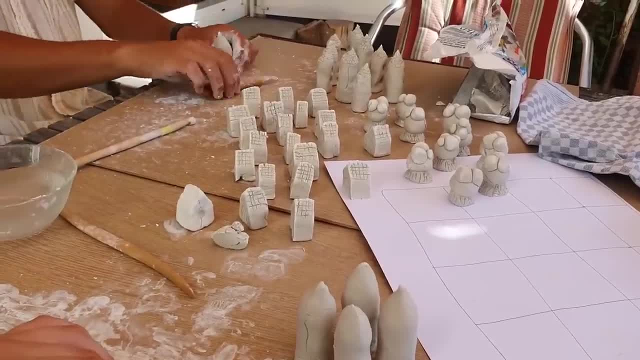 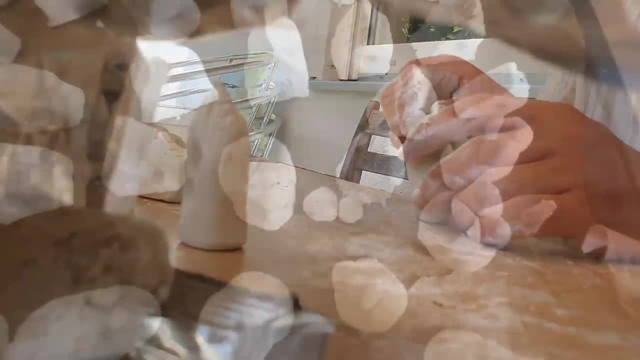 then 10 houses and 10 towers for each player. A total of 50 figurines needed to be handcrafted and painted. I thoroughly enjoyed working with clay outdoors. Here we were adding 3D elements to our little board game. Some parts fell off. 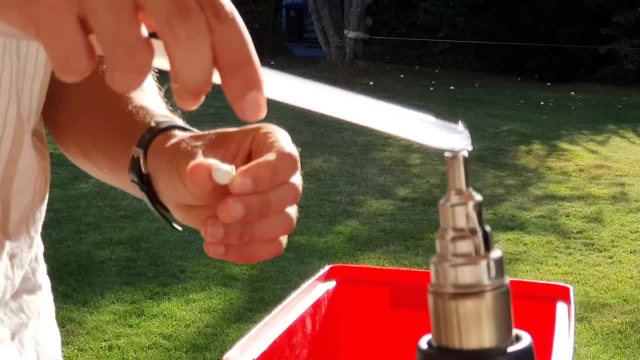 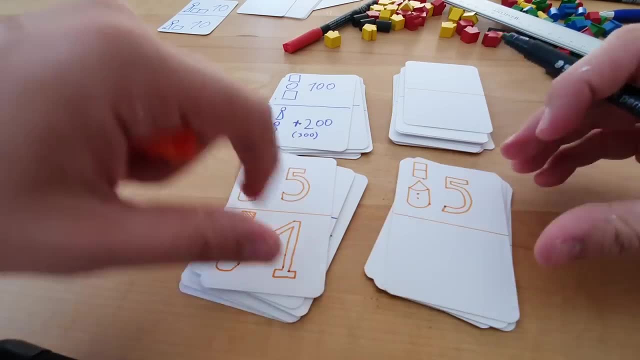 Then glue them back together, then paint them. It's stuck. Then, while we waited for the clay and glue to harden and set, we began polishing the 40 unique cards. Each of us worked on some part of that rather long and tedious process. 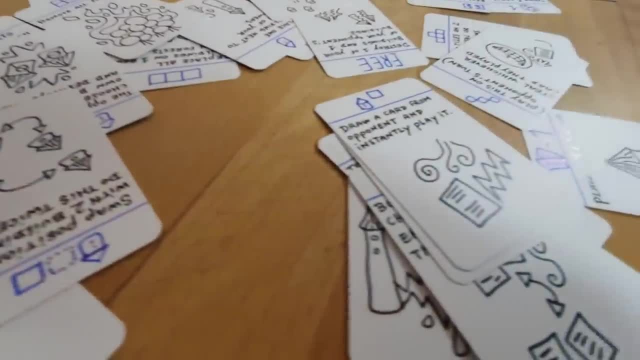 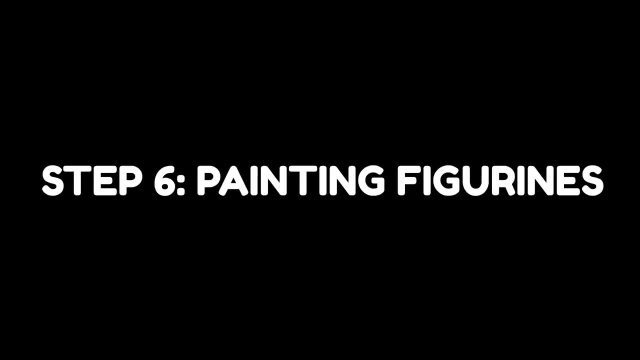 from rewriting everything in a nice chunky font, creating simple and consistent icons for the cards' costs, without forgetting, of course, to add a mini design to illustrate each card effect. Finishing out the painting of our figurines for our board game, Things took a lot longer than expected. 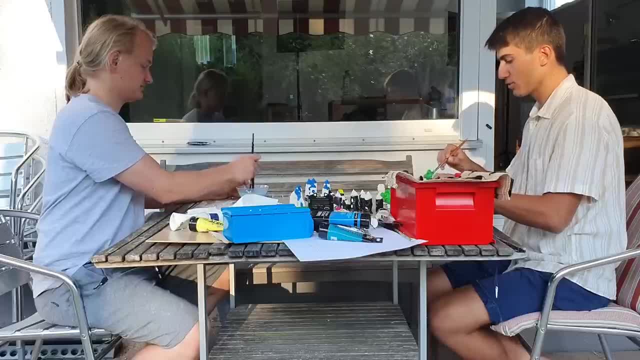 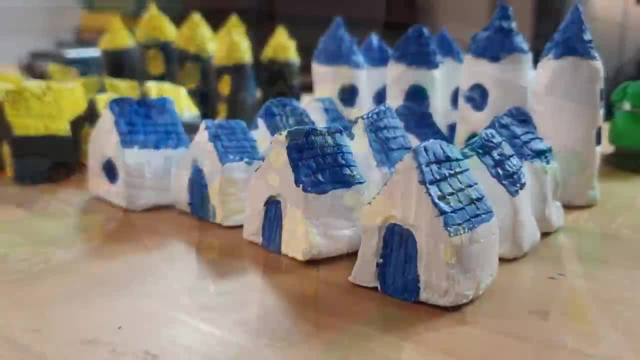 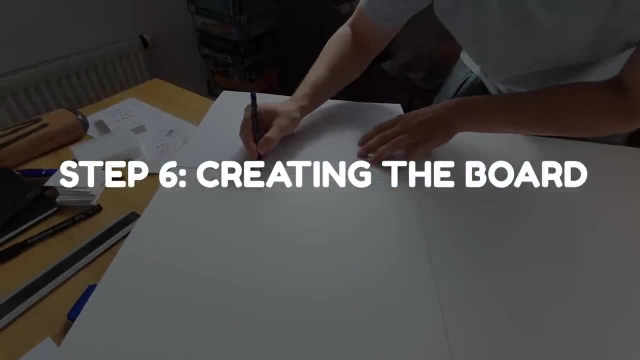 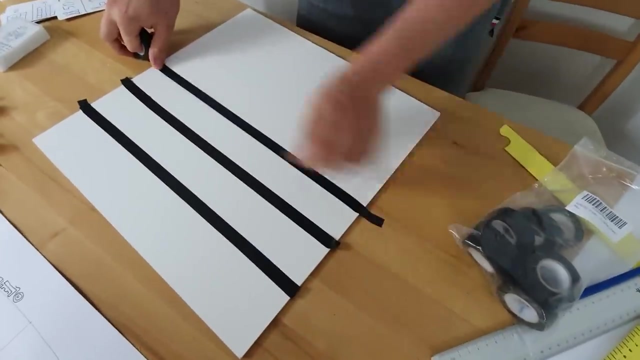 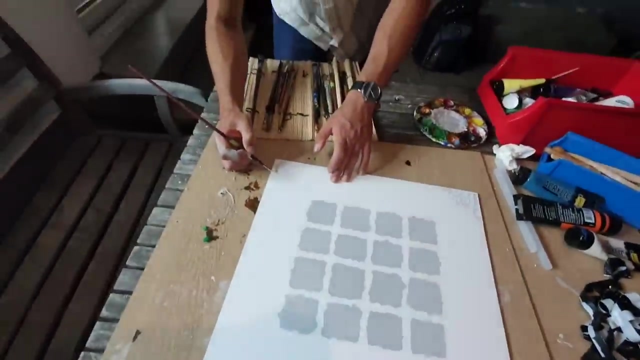 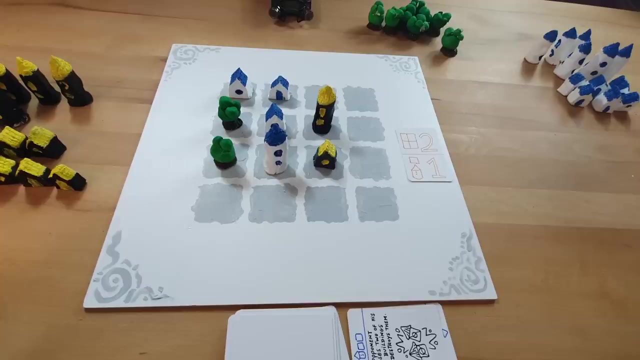 Yeah, I didn't see the sun starting to set, So we've been working for almost 12 hours, Hahaha. Yes, No one in charge of doing art things, of course. No. control Z? No, there's none. Before the last part of the video where Jonas and I play a complete session of our board game. 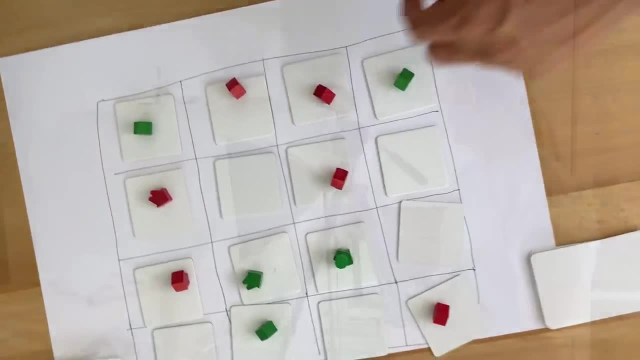 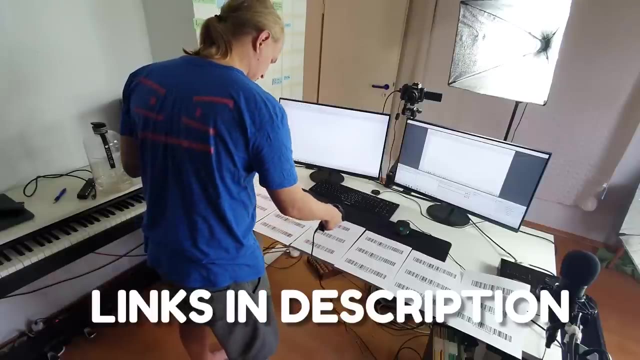 Townshift, I wanted to thank you for checking out the dev blog, and I also highly recommend that you subscribe to both channels, since we created three other completely unique experiments- Links in the description. Alright, let's now get down to the final playtest. 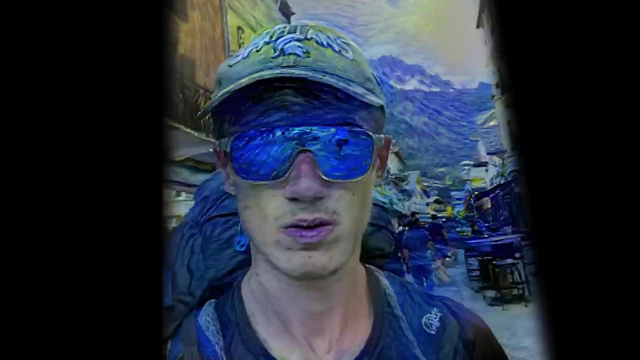 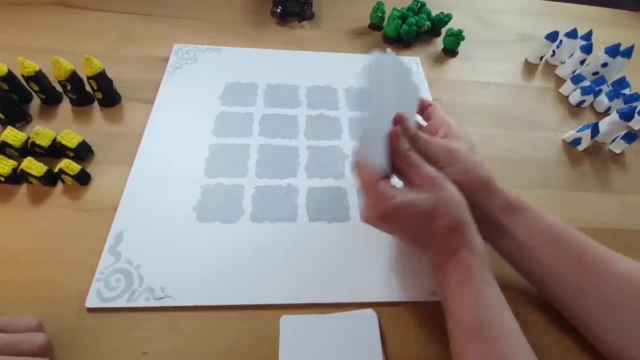 Who will win And who will design the ultimate wizard town. Alright, so we've got our deck of cards. Okay, and here I have the deck of objectives. Yeah, a point system basically Looks quite nice, So, yeah, let's just draw a random one. 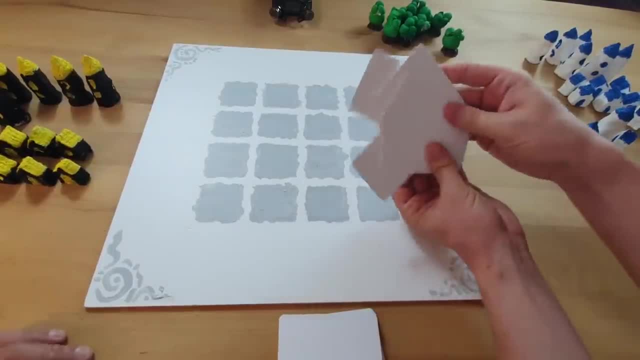 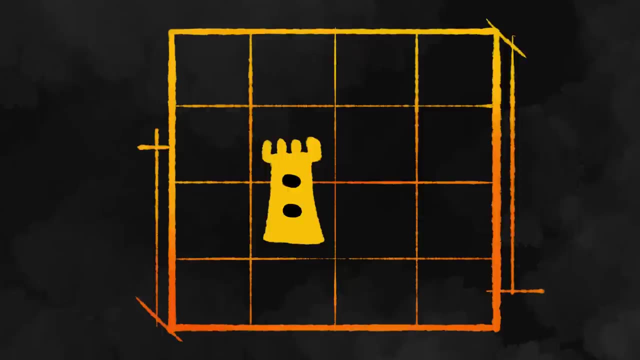 See how we earn points for this particular game. Alright draw one, Alright interesting. So we get two points per square like a layout of four, basically houses, And also when we get one tower it ages into any building. 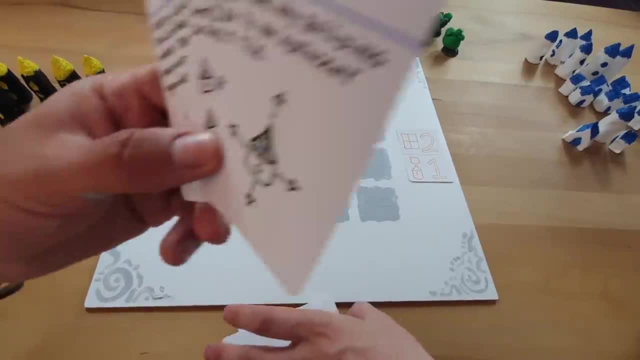 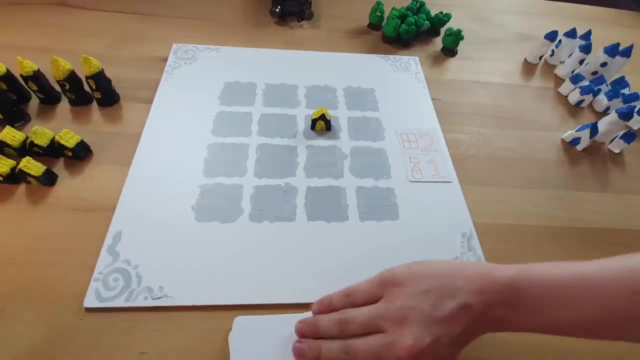 Alright, I'll put that here. And so Everywhere takes three cards. I've got three cards in hand. Let's say I start, And so first thing I need to do is place a building. Yeah, Place it here. I'll draw a card. 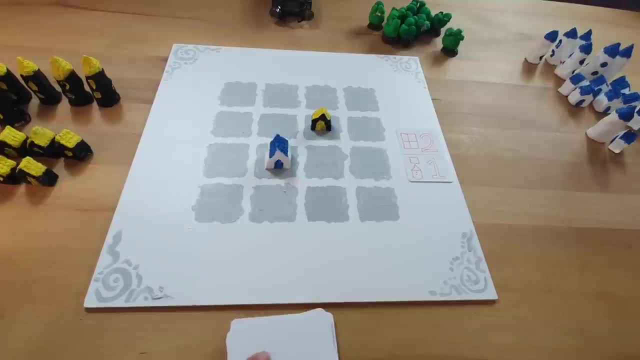 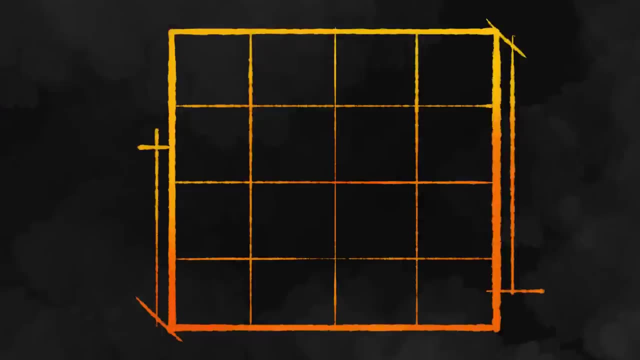 Yeah, And I'll place a building here, Fair enough. I'll draw a card too And remind the viewers, Jonas, how the game ends. The game ends either when all of the tiles on the map are full or if this deck runs out of cards. 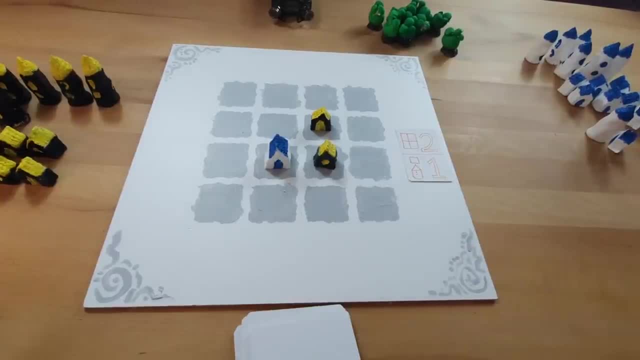 Draw a card. Draw, yeah yeah, Great that you reminded me of that. I'm gonna place a building here. I've got some good cards. I like it. I'm just gonna place a building here and pass on to you. 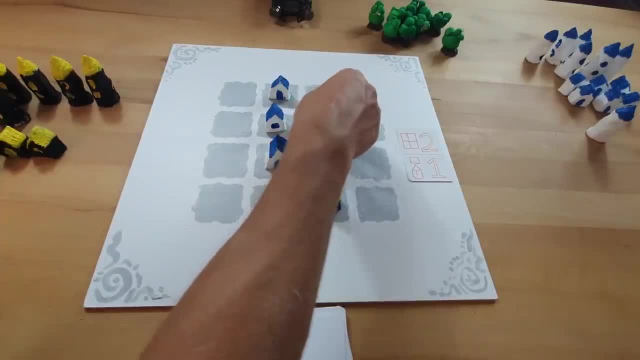 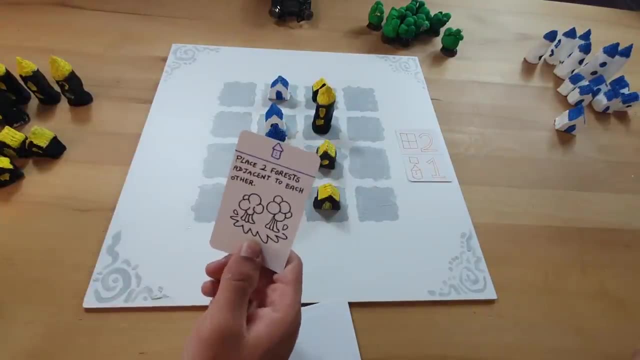 As you can see, the beginning of the game was pretty even, each of us keeping our precious cards waiting for the right moment to pounce Building here, and I'm gonna play this card here, which actually it requires me to have at least one tower. 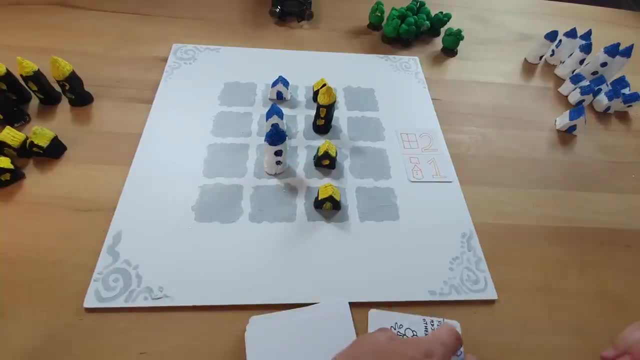 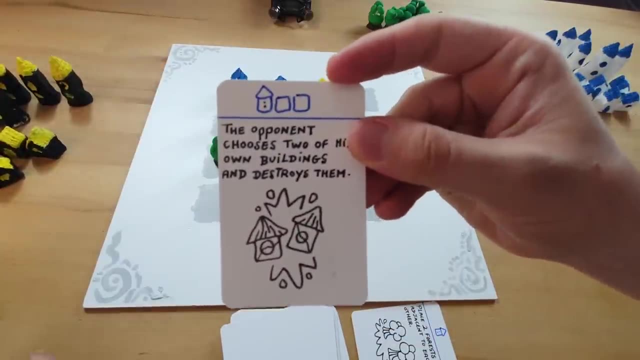 and I can place two forests adjacent to each other. Okay, perfect. And here, Okay, kind of. here The opponent has to destroy two buildings, but you can choose which ones. Oh, that's nasty. Yeah, Oh, that's a really nasty card man. 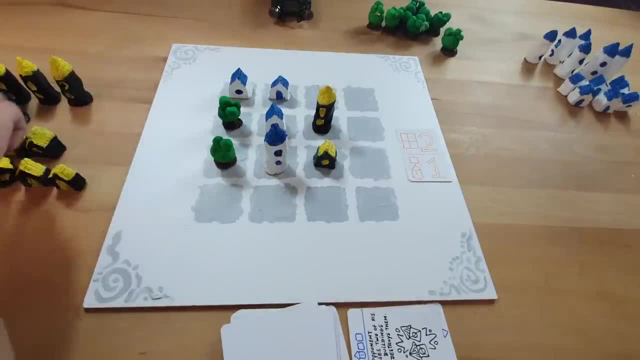 Yeah, Oh, kind of destroying. That is nasty. Okay, I like this one. So I want to build here and I want to play this free card and basically let the opponent decide where you build the building. So I'm more or less caught up. what I lost? 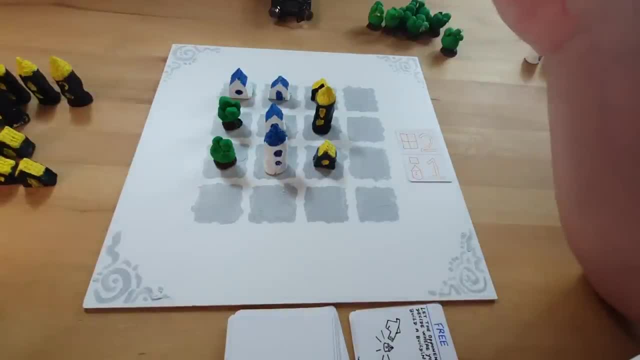 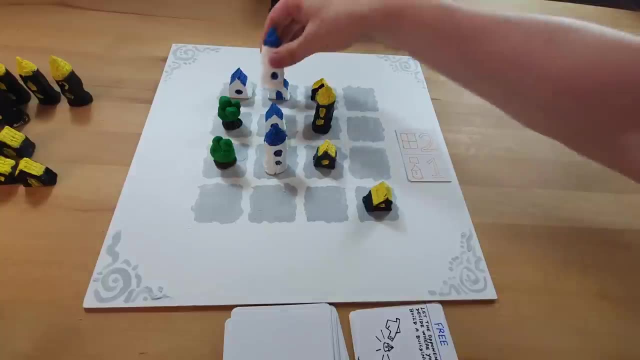 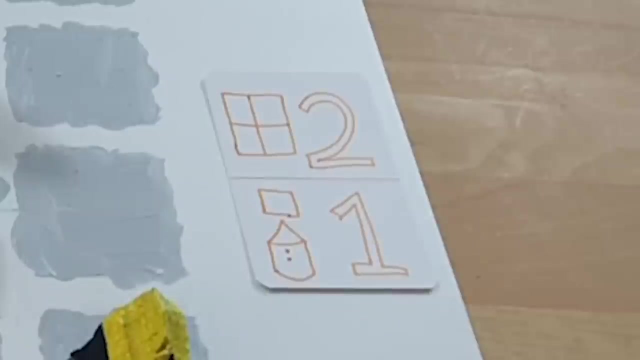 Okay, so I can place one of your buildings, Yep, Here. Okay, I have so many cards in my hand, Lots of options here. They're really. Upgrade this to a tower. Yeah, good one. Keep in mind that each of us is playing with this all-important score system in mind. 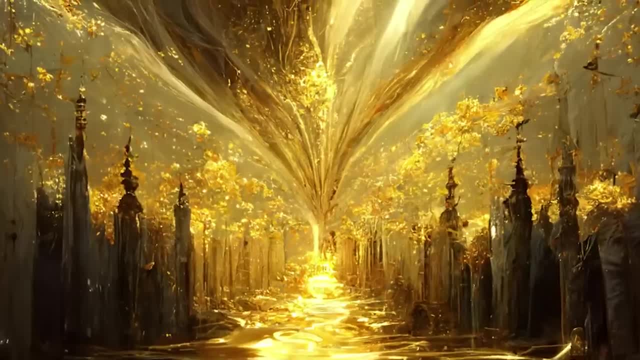 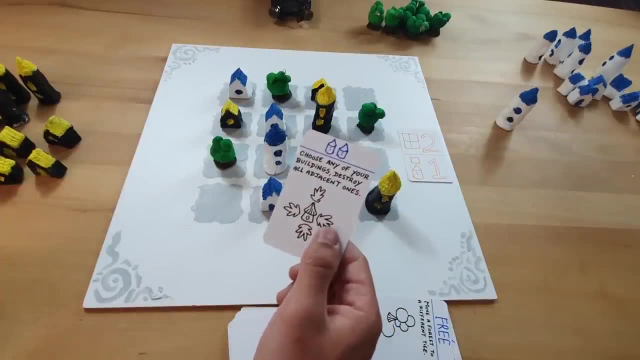 We really need towers and two by twos to score points and hope to win. What kind of card do you have now? It costs two towers and you choose any of your buildings to destroy all adjacent ones. Oh no, Destroy these two here. 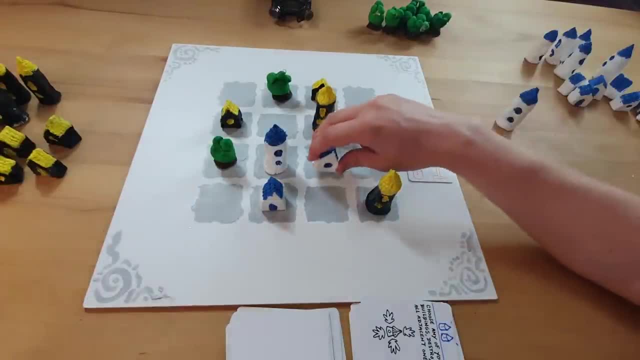 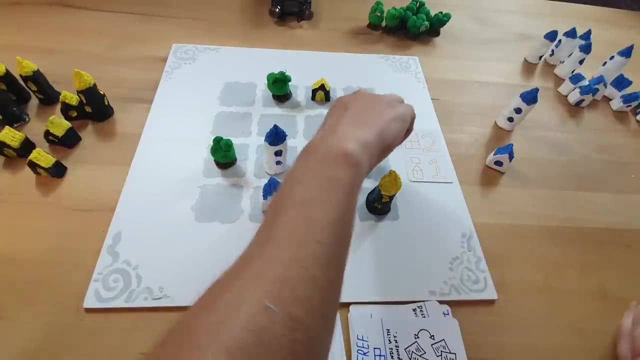 What are you doing to me? Yes, Placing one house here, Discarding two cards to destroy an entire row. I'll get rid of these two. Okay, fine, Just free action. Move any building to any, just tile In here. 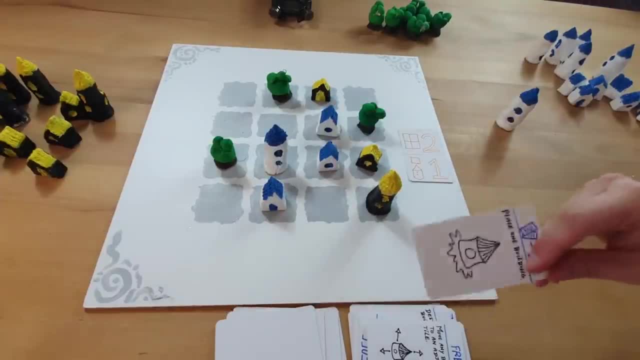 Yeah, Just place one building card. He's got a square. guys, Yeah, He's got a square. I got two points. Now would be a good time for me to end the game. Remove a card from my hand, Move one row by one. 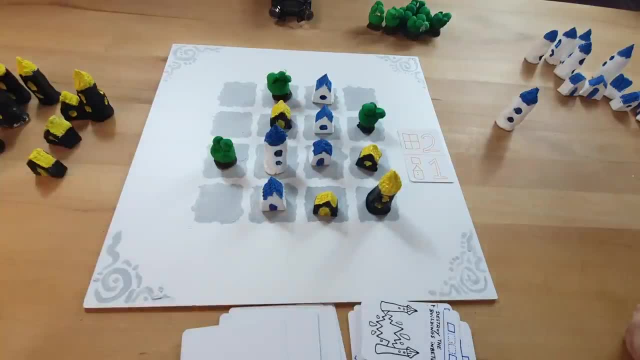 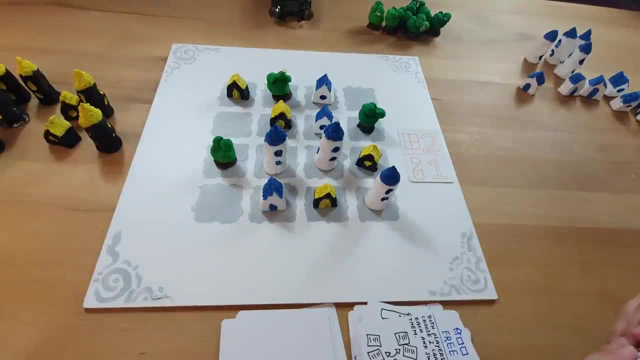 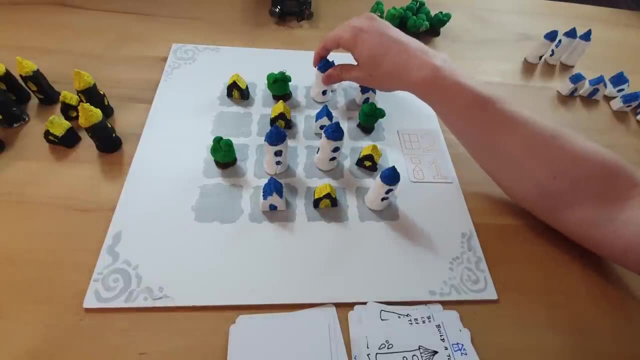 Oh shit, Okay, place one here. Oh, build a tower. That's nice. At this point, Jonas is clearly winning. He has more towers, each scoring him points. We'll end it. Yeah, And I will end it. I'll end the suffering.